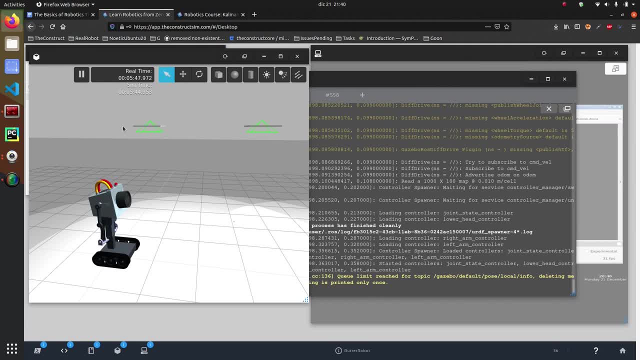 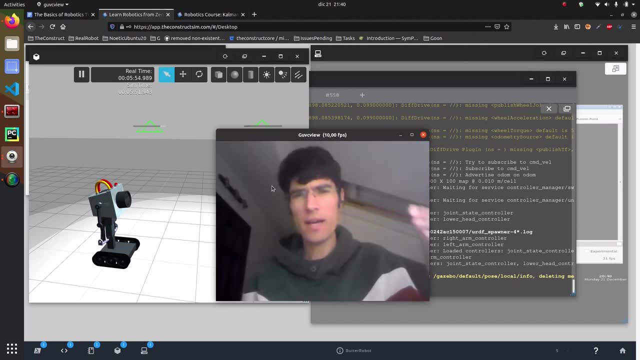 this robot and we have a sensor and sensors have. sensors have always some noise, some kind of noise. sometimes it's really high and sometimes it's really low. it depends on the quality of the sensor and also in the environment. robots in environments like radioactive environments will have a lot of noise. 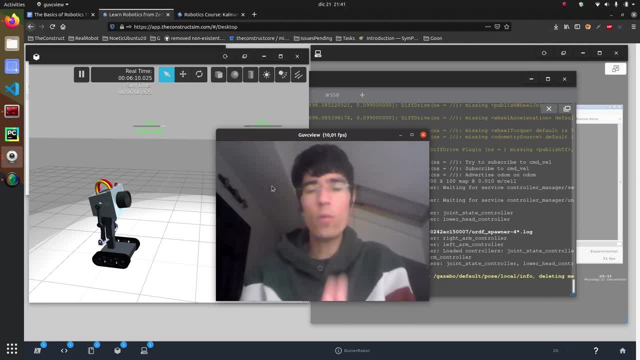 and therefore your algorithms have to cope with this. So Kalman filters allow you to lower all that noise, removal that noise and know what is happening in that sensor. Is it sensing it? is there something on top of this robot or isn't? So the basis of Kalman filters are: 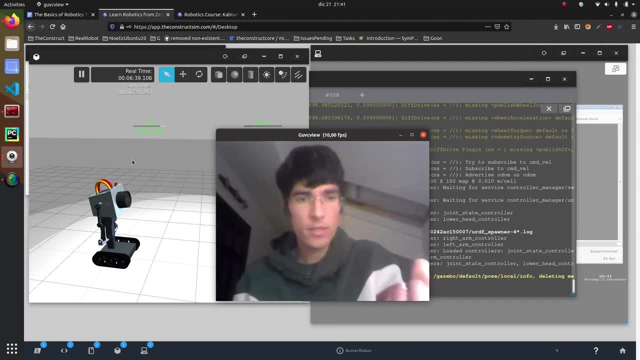 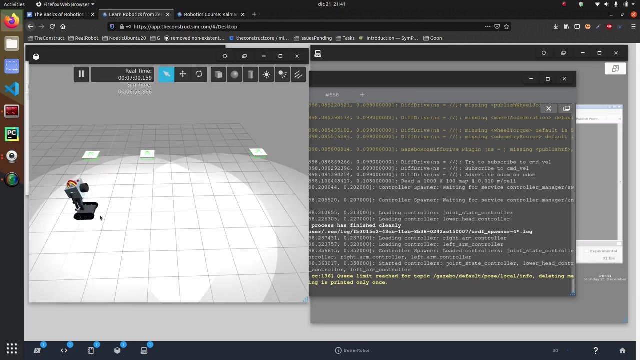 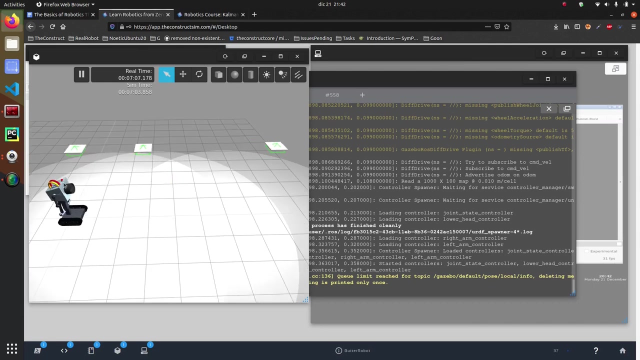 Bayesians filters, which essentially Kalman filters, is a subgroup of them and we're going to implement here right now one of them to allow the robot to know where he is in this scenario. So the robot is going to move forwards, only forwards or backwards, and it has to know based on the readings. 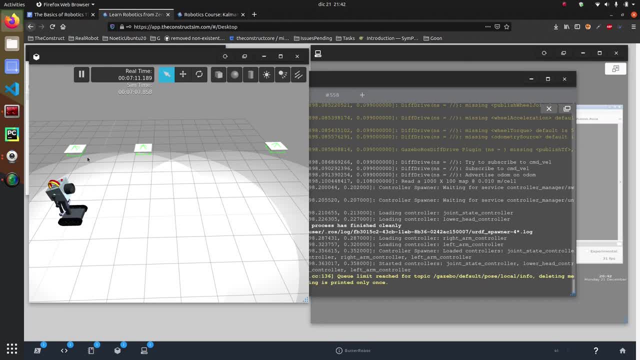 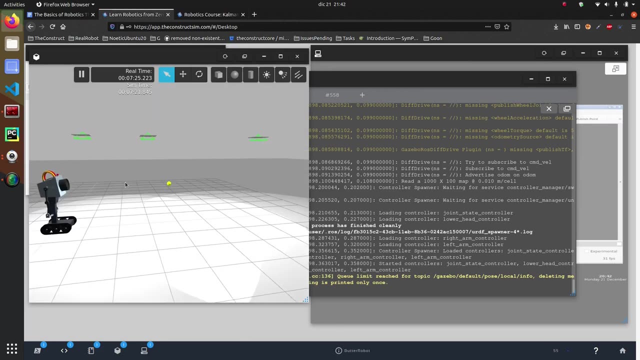 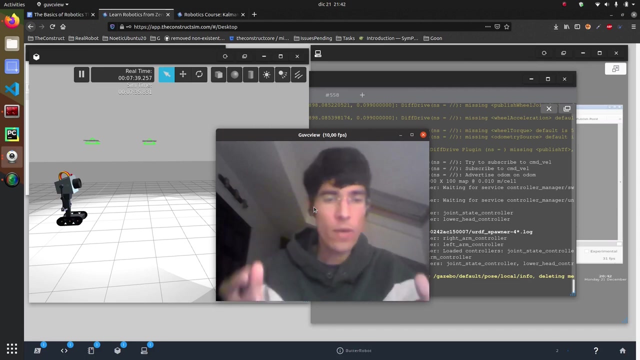 of this sensor? where is? where is he so is? is he in line zero, line one, line two, line three, line four, five, six, seven, eight, nine? so, depending on where he is, he will have readings or not and, based on this asymmetry, at the end he will learn. he will learn in some way. 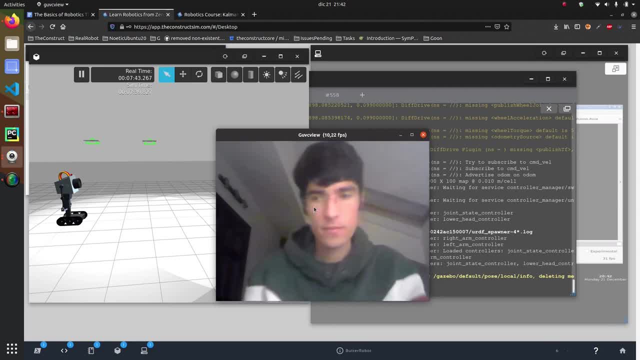 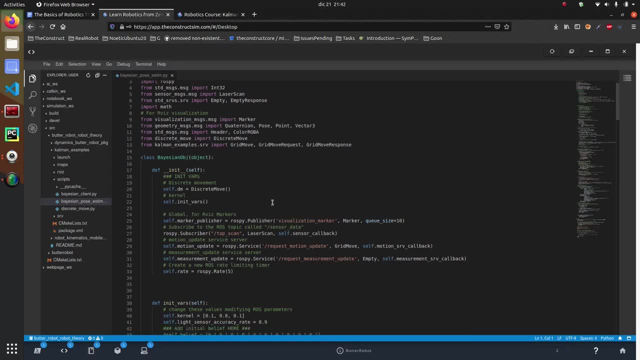 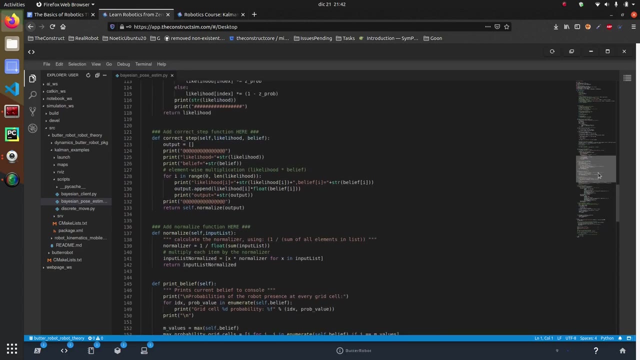 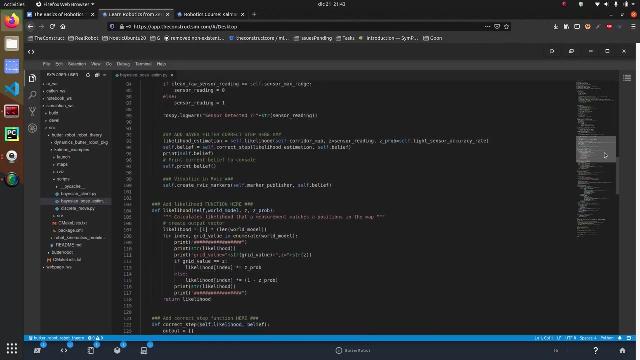 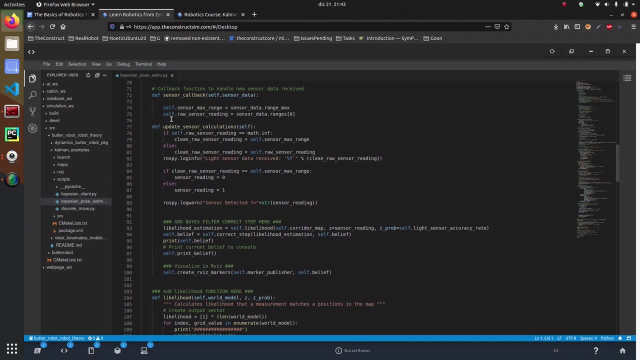 where he is. So let me, let me just show you a bit the code. So Bayesians, basically, are made of two things. they are made of a prediction state and a correct state. so let me show you here. so this is where we update the. 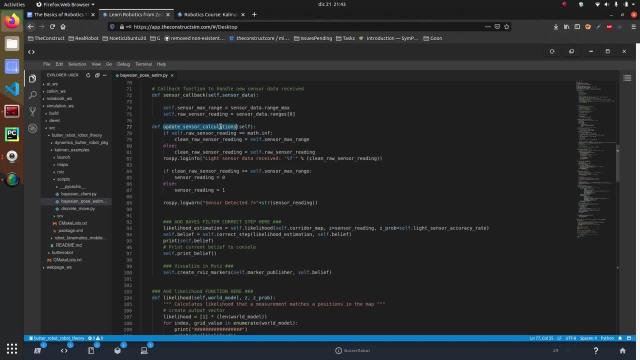 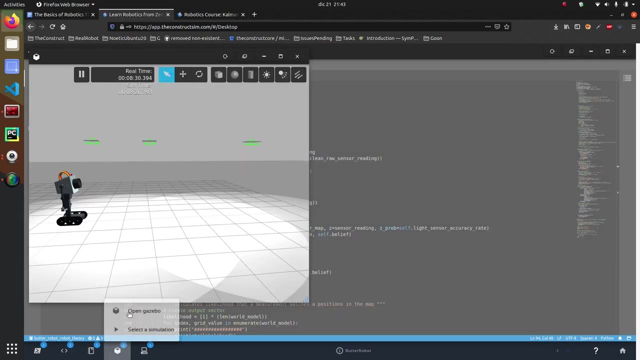 sensor and we make the calculations based on the sensor. okay, and here we correct it. We make a belief based on the sensor. so is: am I reading this, am I seeing this, this light here, or not? and based on that, we can say that if I have a reading, if it's- 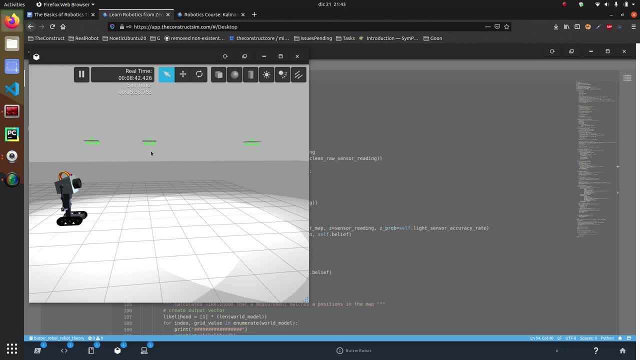 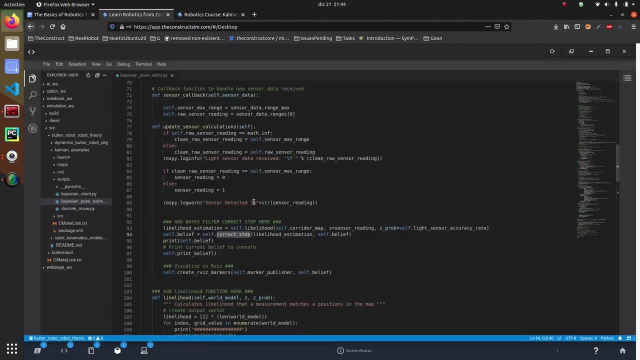 detecting something, I have to be here, here or here. if I'm not, then I have to be here, here, here and all this section and here. so, based on that, we know if it's in one of these three places or or not. based on the sensor. okay, then there's the movement phase, so we make a 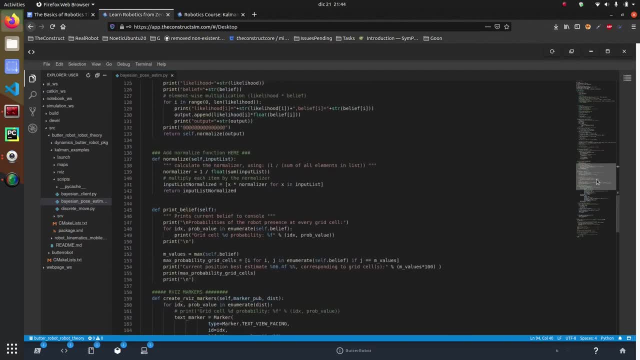 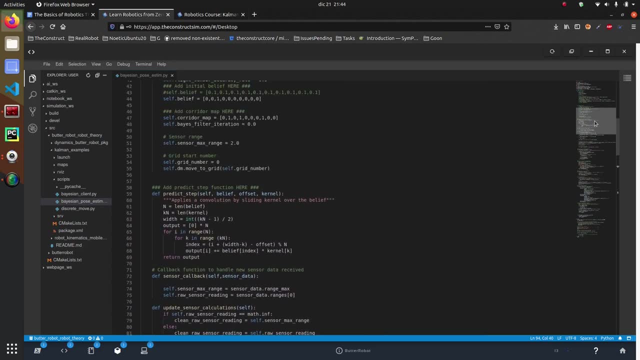 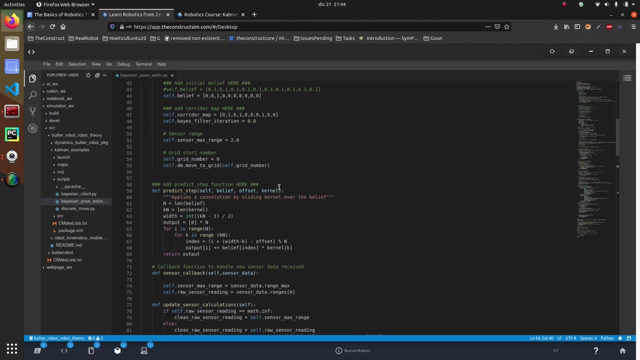 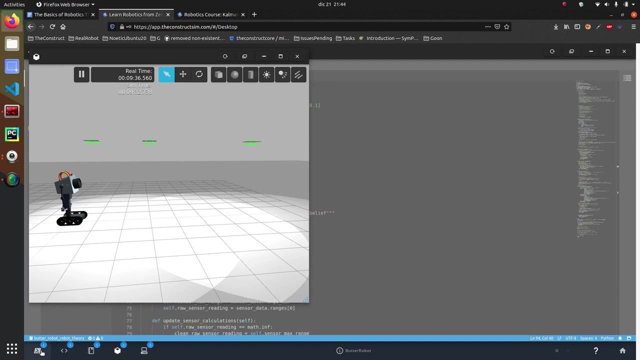 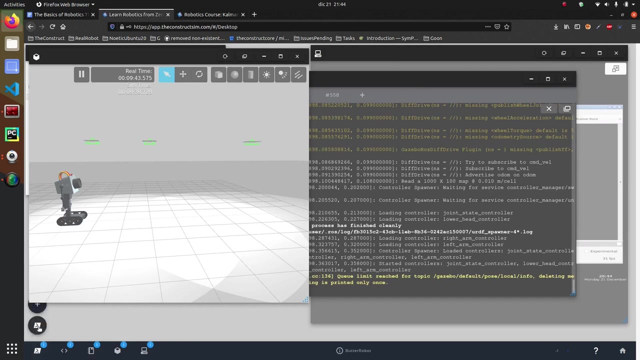 prediction, and that's where we do this. let me just the predict step, and here what we do is cross the, the beliefs with this movement of the robot. so let's have a look how this is working. so I I've created, Here we go. So I'm going to now launch a robot. 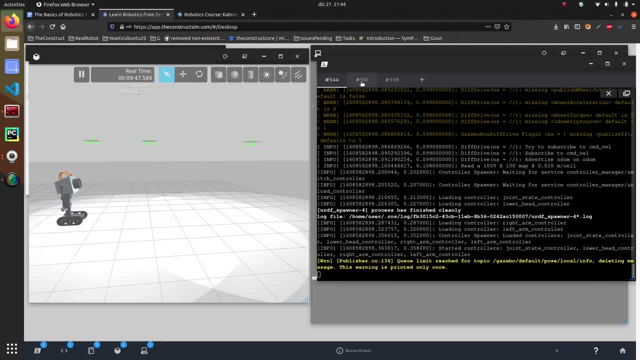 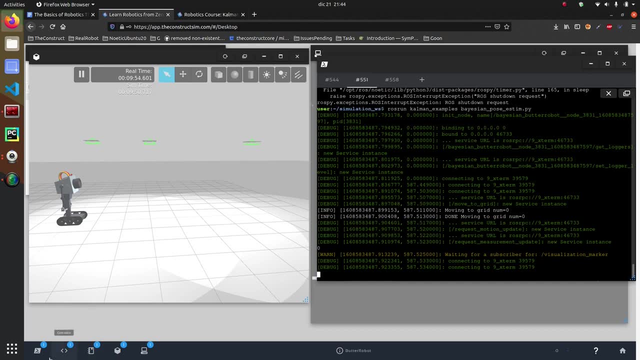 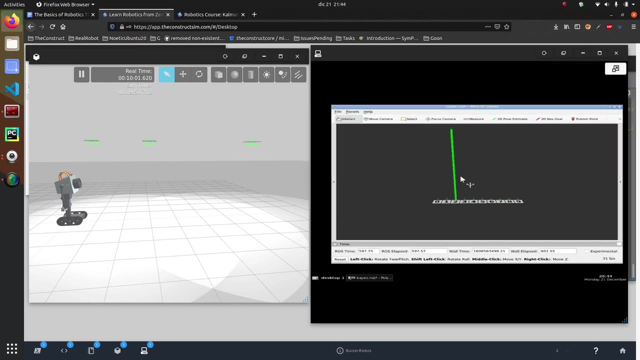 in SageMap. so I'm going to now launch a robot in SageMap, okay, so now we are in launch the Bayesian pose estimate and, if you see, here we have the initial belief. so the initial belief is that the robot is in section 2 in grid 2, which is 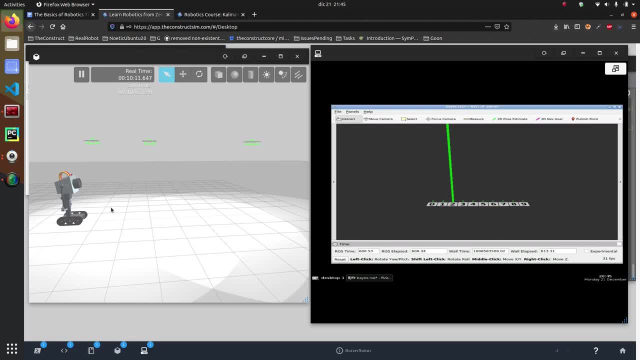 totally random, so I just put that one there. obviously he isn't there, but his first belief is as good as anyone, so we could put this everything with the same probabilities. but I've stated just that that it has 100% of probabilities that he is in number two and, based on the experience, he will lower that and adapt. 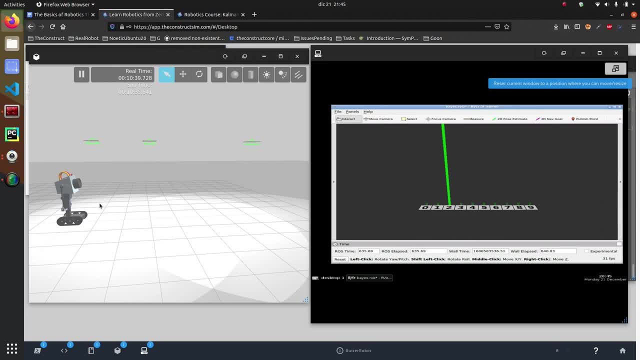 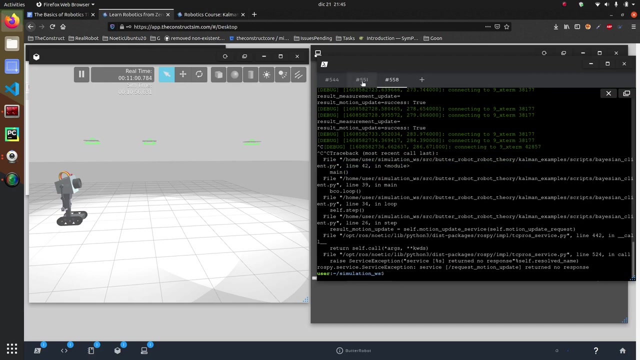 it with this filter, so that at the end he knows in reality where he is based, on the movements that he makes he's done and the readings, the previous readings, that he's done. for that we go here and this system has two services and we will call these two services. 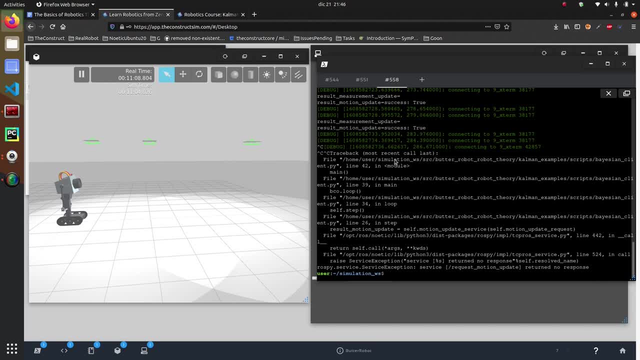 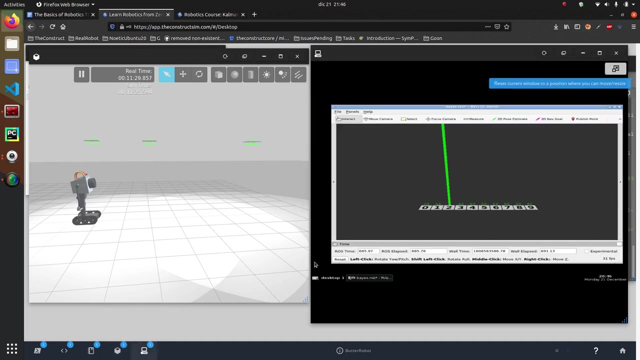 that are for the movement phase and for the sensor calculation phase, and through this feedback- reading the sensors and moving, reading the sensors and moving- we will be able to improve our predictions. so let me just run this. there we go. so now he's making the predictions and, as 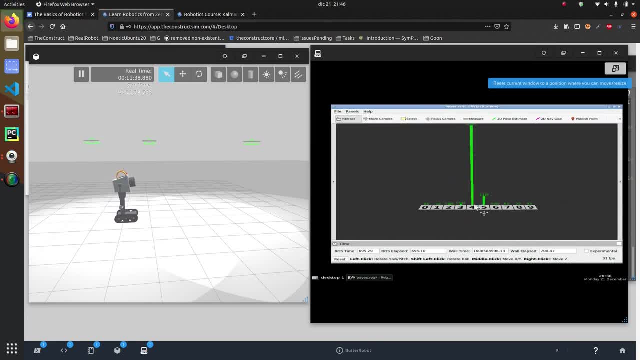 you can see, now we don't have zero here anymore and we can see that he's done now a bit more. he makes the reading again and he says: i think i'm here, but maybe i'm around there, i'm not sure- then again, and because now he doesn't have any readings- 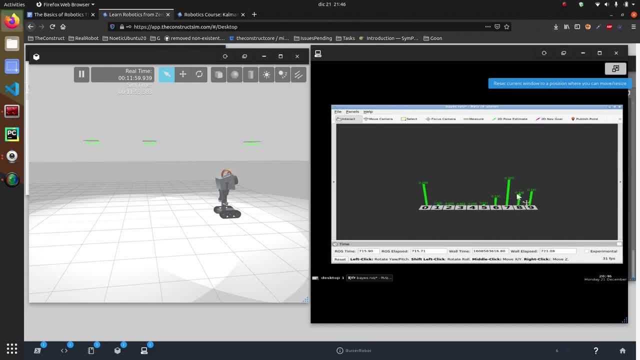 it starts to don't know where he is exactly again, and you can see that it's becoming to stabilize. it doesn't know i'm here or i'm here, okay, maybe he thinks that he's in number two, which he isn't, then again. well then, he got this probability. 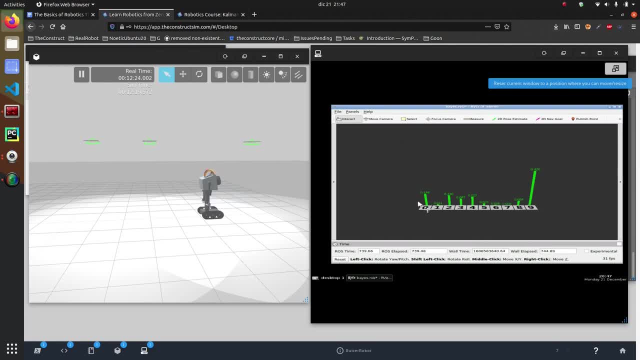 quite right. now we are resetting. so now we're going back again to zero and starting again, and he will do this again, and again, and again until we are happy with the results. you see, now he makes the reading again: movement and reading, movement and reading, as you can see in the first loop. 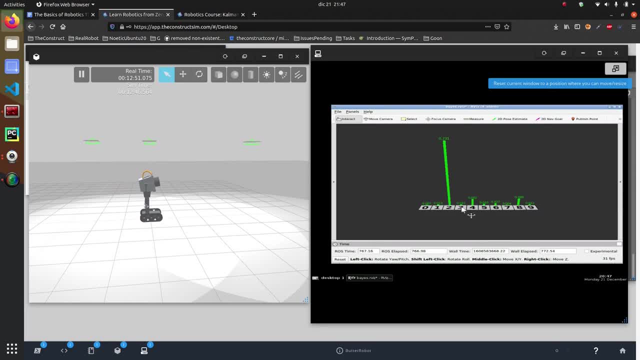 he's getting it right already now. number three and it has like 100 of probabilities now, 80 percent of being in number four, 60 percent along the line because we are moving the probability to go lower because he doesn't have any new sensor data. now you see he got sensor data, so, wow, he's in seven. he knows that. 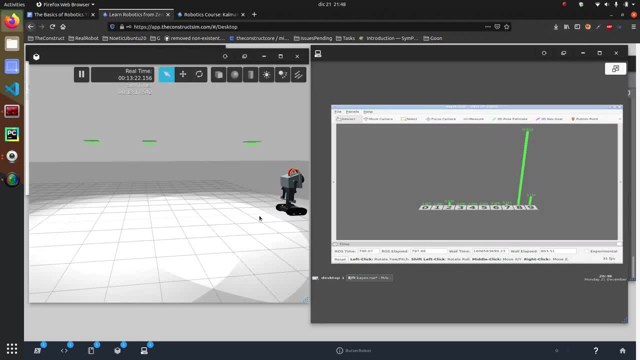 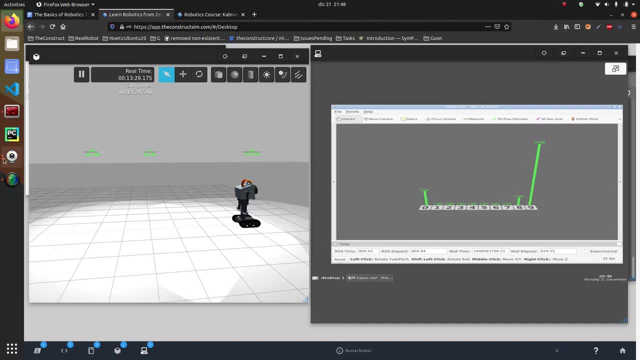 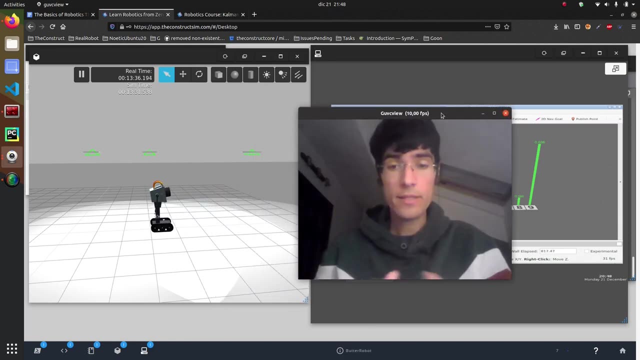 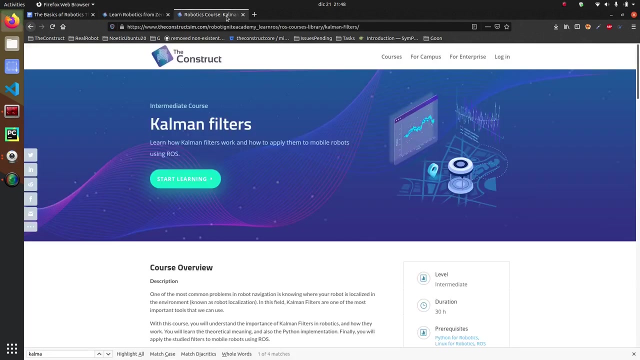 he's there and he said, okay, probably I'll be here now in eight, now in nine and now again, and that's Bayesian filters. so, as you can see, it's very, very simple. in theory it's very simple, but it's the basis to learn loads of stuff. 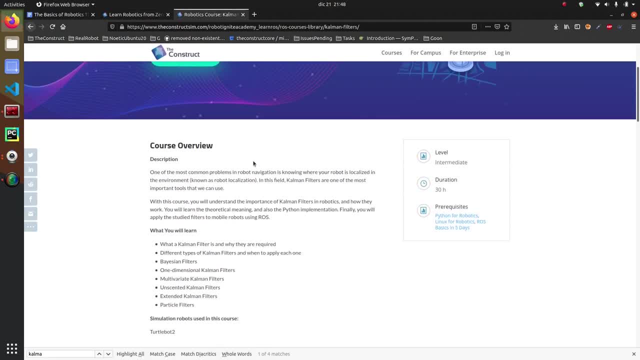 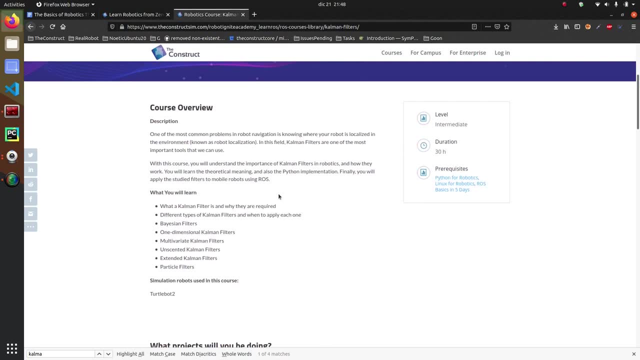 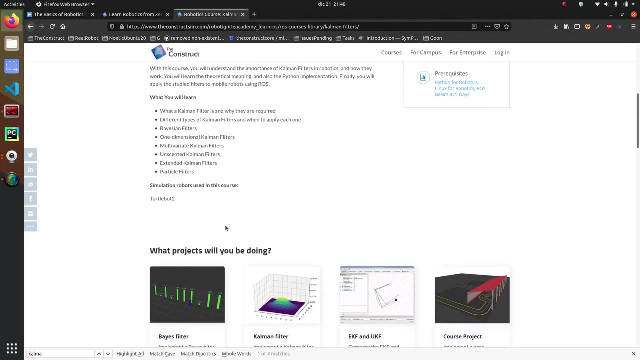 I've learned this. I mean, I didn't know how to implement this in ROS and I did this course, which you can learn most a lot of things, not only this, this is just the tip of the iceberg, and, and so you're going to learn this. so, Bayesian filters. 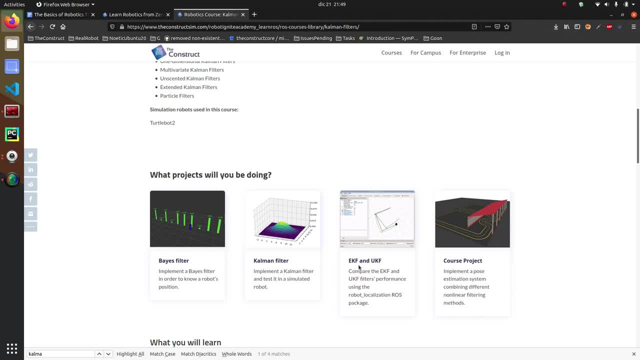 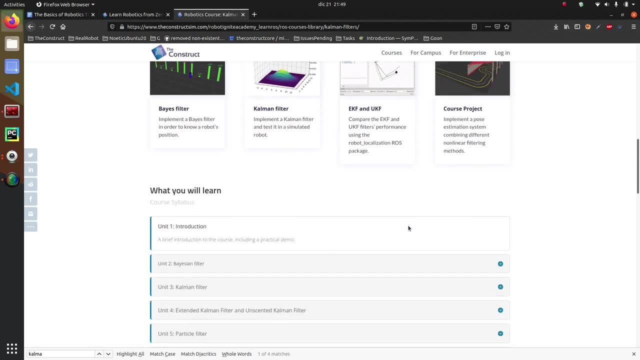 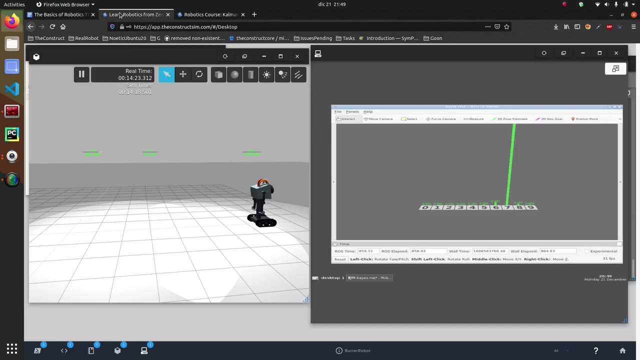 and you're going to learn this. so Bayesian filters, then Kalman filters, EKF and UKF, which are basically ways of doing that, and then you'll have a project. so you'll have lots of things to learn and it's really nice and I really learned a lot with this and I got it working. so, with a 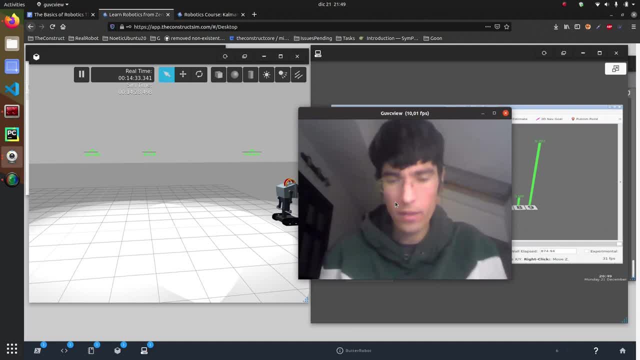 robot- totally different from the course, by the way- so I can guarantee that it works, so that I think that's all for today. thanks a lot for being here. check out the course is really nice- and see you in the next video. peace.